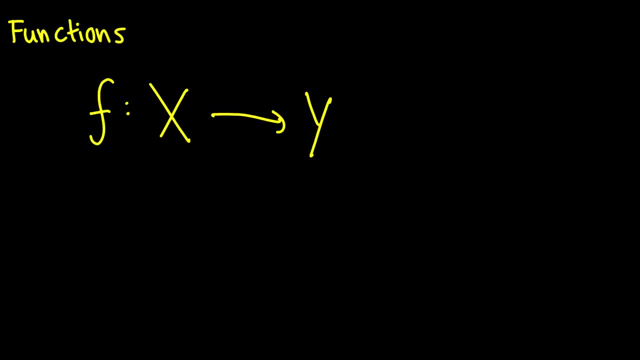 Today we're going to introduce functions. A function looks like this: It is a function f that maps x to y, So x maps to y. There's a bunch of terminology we have to do here, so I'm going to list it here. Everything in the set x is going to be the domain. 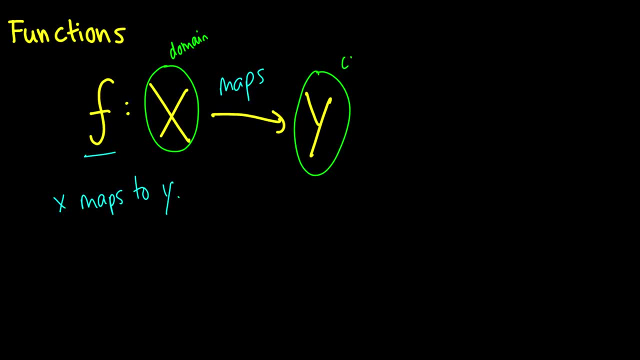 All the elements in the set y are going to be the codomain. And I should introduce another notation you're probably more familiar with: For each of the elements in the big set x and each of the elements in the big set y, we write that f of x is equal to y And all of the numbers 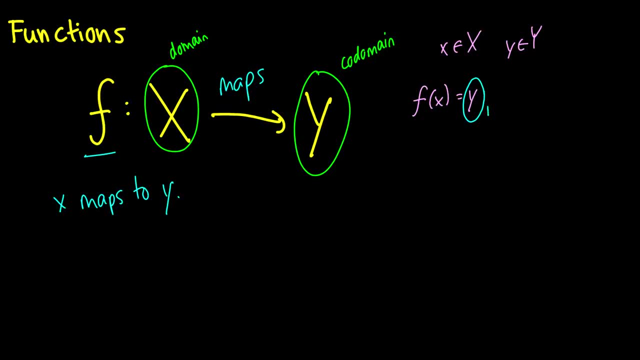 that can be output through the function is called the range or the image of f, So the set of y and y, such that f of x is equal to y. This is the range or the image, And all of the x are the elements in the set x. 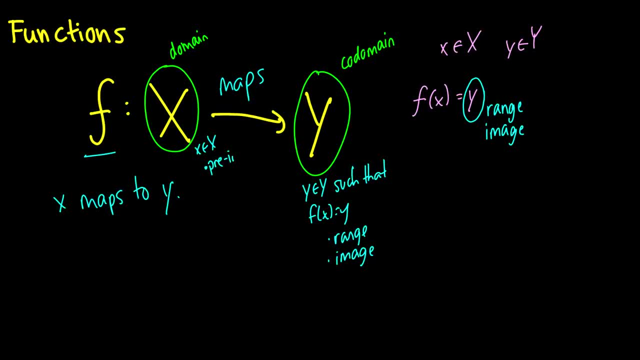 And all of the x are the elements in the set x And all of the x are the elements in the set x are going to be the preimage. So here's a nice function and I've kind of written a lot around it. You might be thinking: okay, I understand, f of x equals y. I don't get. 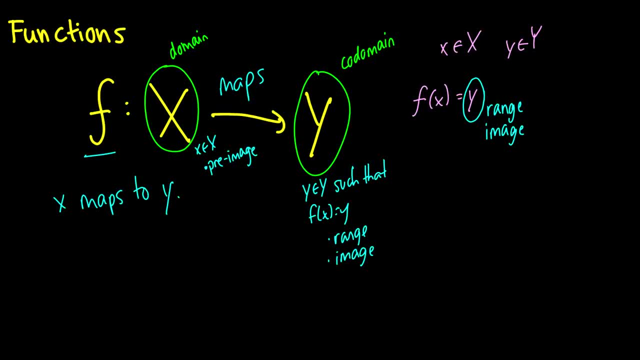 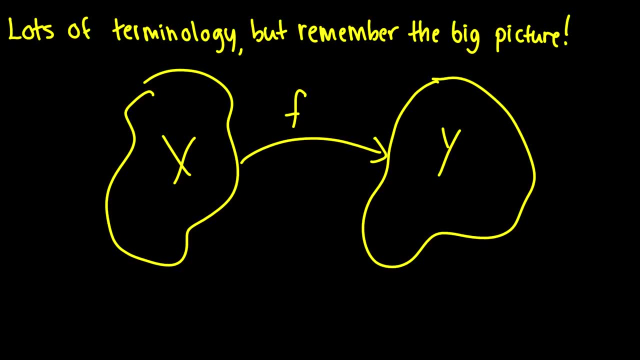 this notation. It's a little bit confusing. So here's a picture, And pictures are good because it kind of shows what we're doing here. So we have a domain in our x's and we have the codomain as the set y. Now what we do is we take an element. 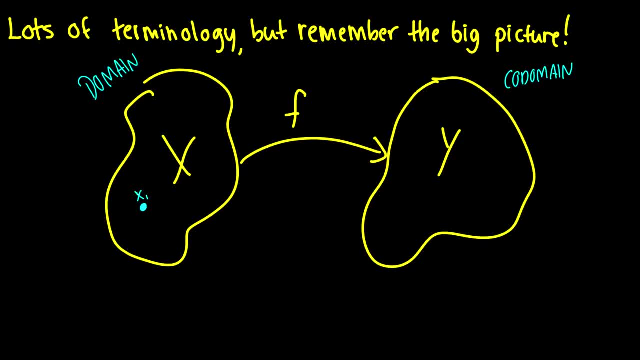 in x, so let's call this x1, and this function f takes this guy and plants him somewhere in here, which we'll call f of x1.. So this function simply maps this guy in x into some other set of x's. So this function simply maps this guy in x into some 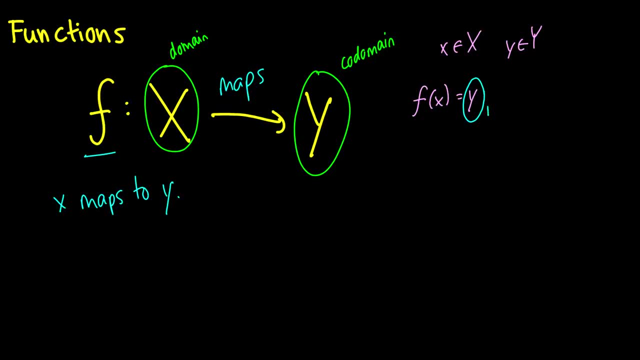 that can be output through the function is called the range or the image of f, So the set of y and y, such that f of x is equal to y. This is the range or the image, And all of the x are the elements in the set x. 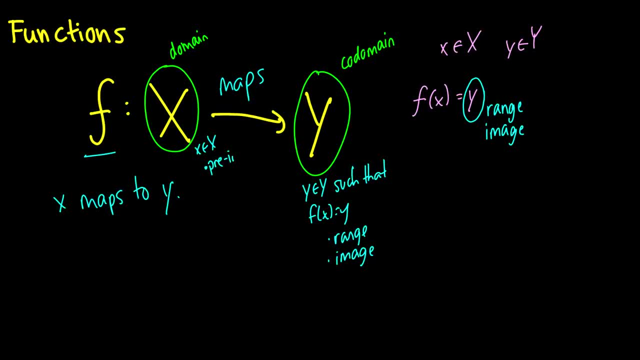 And all of the x are the elements in the set x And all of the x are the elements in the set x are going to be the preimage. So here's a nice function and I've kind of written a lot around it. You might be thinking: okay, I understand, f of x equals y. I don't get. 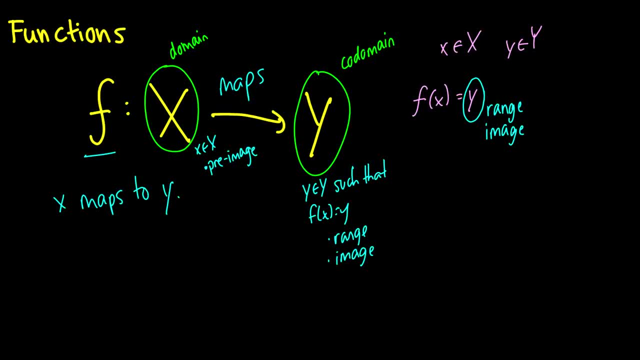 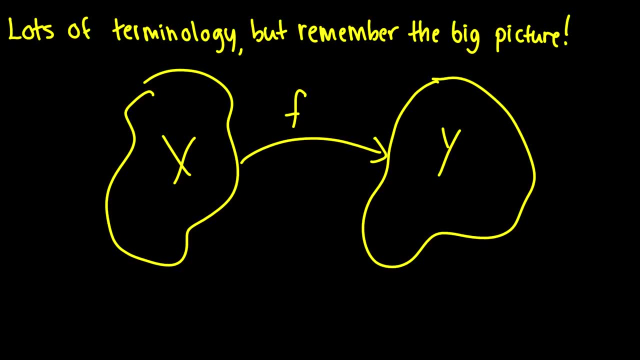 this notation. It's a little bit confusing. So here's a picture, And pictures are good because it kind of shows what we're doing here. So we have a domain in our x's and we have the codomain as the set y. Now what we do is we take an element. 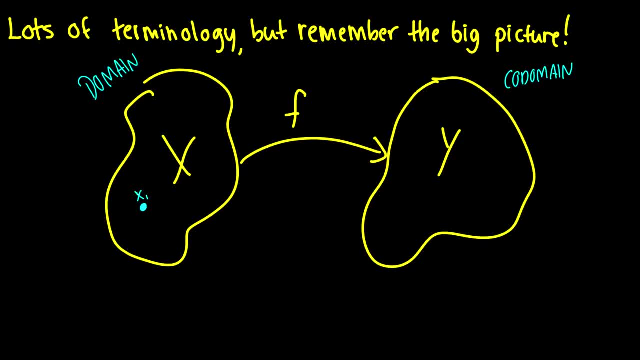 in x, so let's call this x1, and this function f takes this guy and plants him somewhere in here, which we'll call f of x1.. So this function simply maps this guy in x into some other set of x's. So this function simply maps this guy in x into some 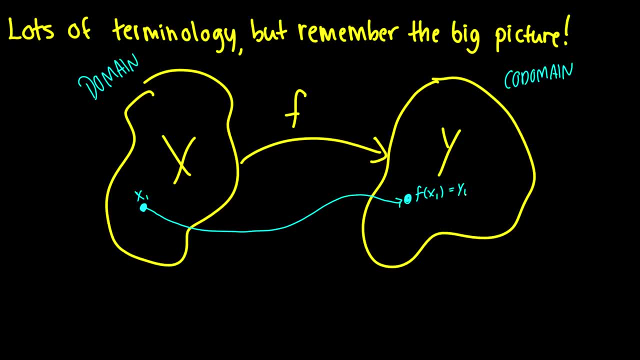 other guy in y And we'll just call this guy y1.. And of course this is the function f. so f maps all the little x in x to a little y in y. And what we do here is, let's say, no matter where we take our guys here, it's always going to be mapped on to some other guy in. 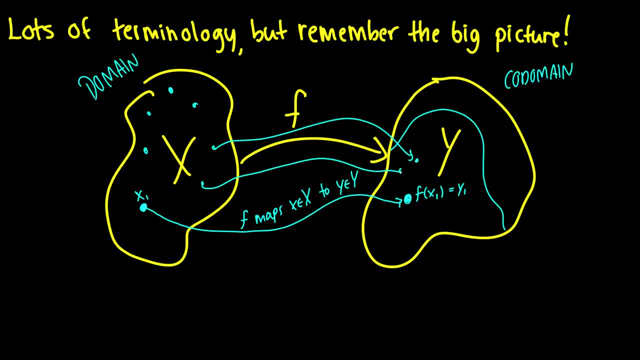 x, And we'll just call this guy 0x, And the only way we're going to be able to get to that is that f nochmal gives us some object in this lower space. So what we call this lower space, where all the objects are right in here, is going to be the range And all. 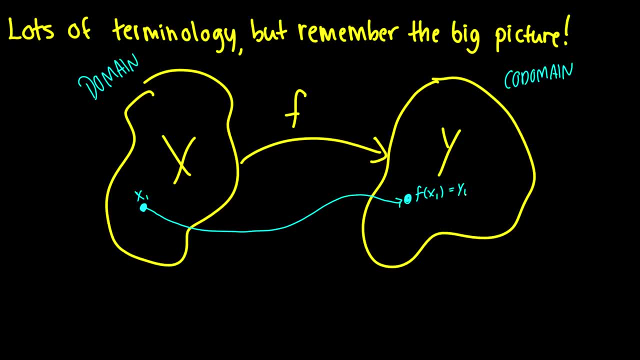 other guy in y And we'll just call this guy y1.. And of course this is the function f. so f maps all the little x in x to a little y in y. And what we do here is, let's say, no matter where we take our guys here, it's always going to be mapped on to some other guy in. 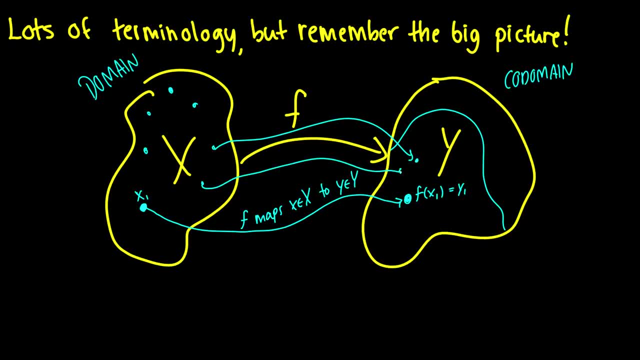 here. So f maps some object in this lower space. So what we call this lower space, where all the objects are right in here, is going to be the range, And all this stuff up here in the red zone that can never be attained is part of the codomain, but it's. 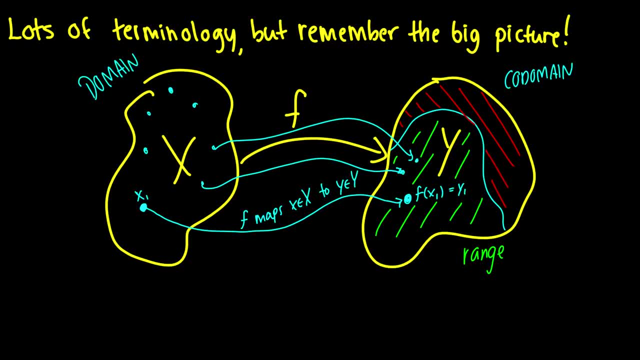 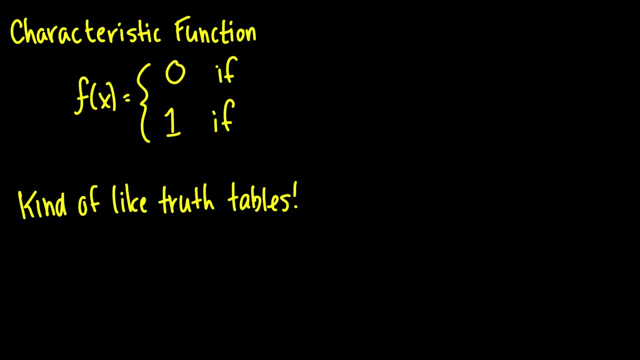 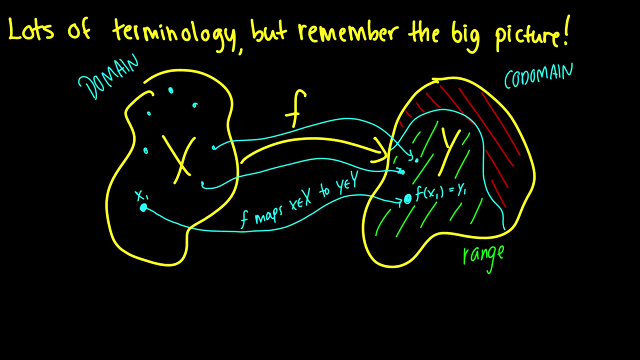 not part of the range, since the range are all the things that f can take elements in x to. so again, this is a little bit more abstract than you're probably used to dealing with functions, but hopefully in an example will make this very, very simple. unfortunately, I don't have a nice example written, so we're going to do one. 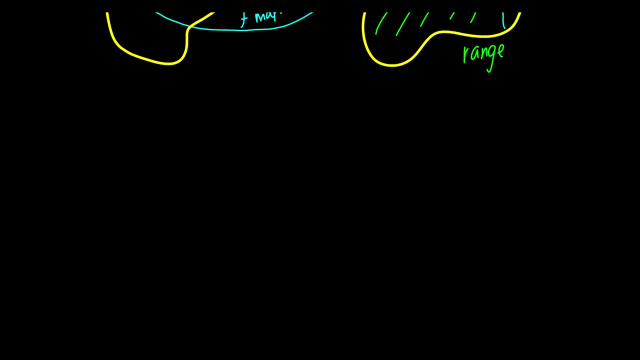 off the top of our heads here. we all know the function f of X is equal to x squared. so let's say, we're working in integers, we're just going to work in integers. so what we can do is we can draw out our little thing here and we 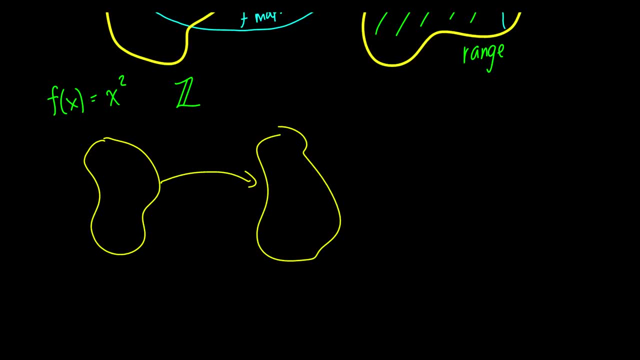 can draw out a little thing here and we can do our nice f function. so let's take the number one. okay, actually, let's not do that. let's take the number two, because two is a better. first example what this does is this: maps it onto some spot f of two, and when we plug two into, 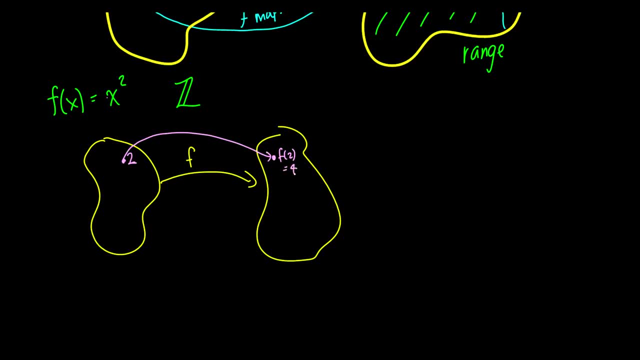 our function, we see that this is equal to four. okay, so then we come here and we say, well, what about zero? now, this one's pretty easy, this just maps on to zero. now, what about, I don't know? let's say four. well, four maps on to zero. 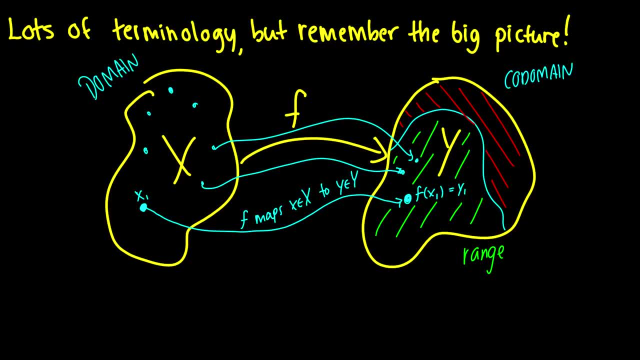 this stuff up here in the red zone that can never be attained is part of the codomain, but it's not part of the range, since the range are all the things that f can take elements in x to. so again, this is a little bit more abstract than you're probably used to. 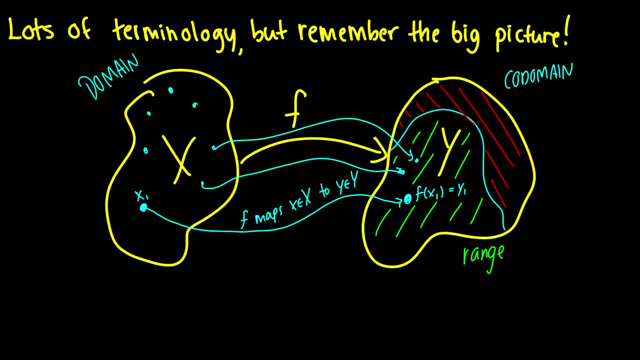 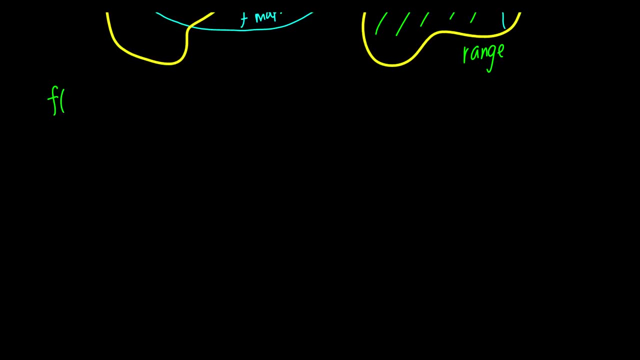 dealing with functions, but hopefully in an example, will make this very, very simple. unfortunately I don't have a nice example written, so we're going to do one off the top of our heads here. we all know the function f of X is equal to x squared. so let's say we're working in integers, we're just going to work in. 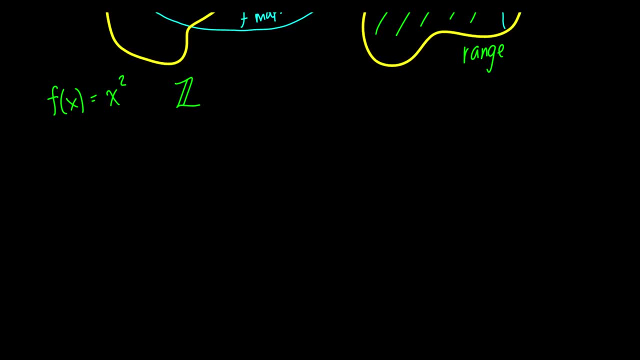 integers. so what we can do is we can draw out our little thing here and we can draw out a little thing here and we can do our nice f function. so let's take the number one. okay, actually, let's not do that. let's take the number two because 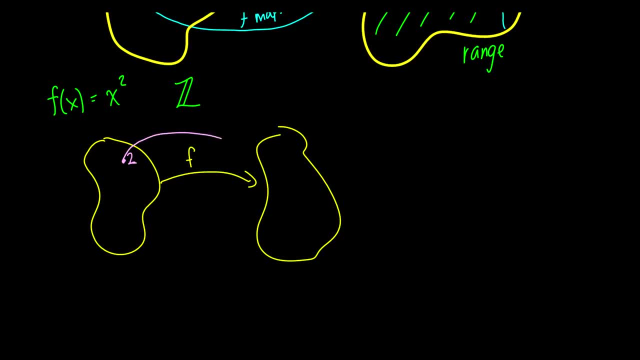 two is a better first example. what this does is this maps it onto some spot f of two, and when we plug two into our function, we see that this is equal to four. okay, so then we come here and we say, well, what about zero? now, this one's pretty easy. this just maps on to zero. 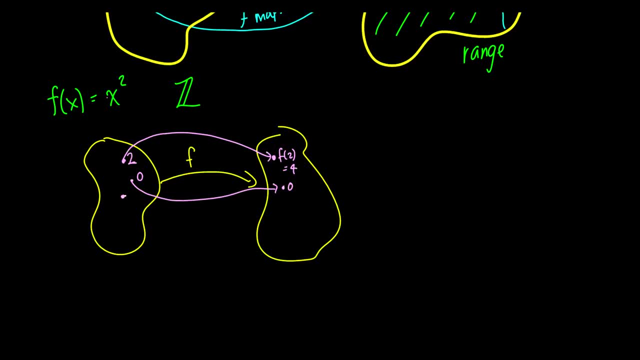 now, what about, I don't know. let's say four: well, four maps on to zero. well, four maps on to zero, over here to the number 16. so this seems pretty good, and because it's all integers, what we can do is we can say: oh, what about negative four then? and here's: 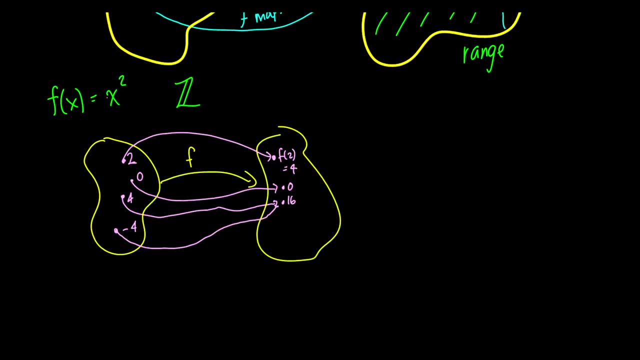 what's interesting is that this maps on to the same point. so if we say that X is an integer and Y is an integer, then what this function does is it maps an integer to the same point. so if we say that X is an integer and Y is an integer, 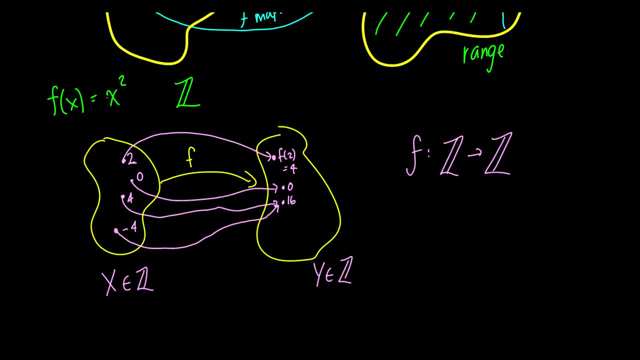 we get. what we're saying is that this maps an integer onto another integer. but what's more interesting really is that it doesn't just map an integer onto an integer, it maps any integer onto a positive integer. so that's a little bit interesting. we have a function that takes an integer into a positive. 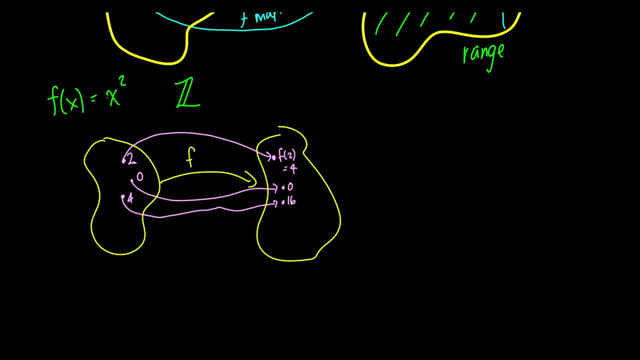 well, four maps on to zero, over here to the number 16. so this seems pretty good and because it's all integers, what we can do is we can say, oh, what about negative four then? and here's what's interesting is that this maps on to the same point. so if we say that X is, 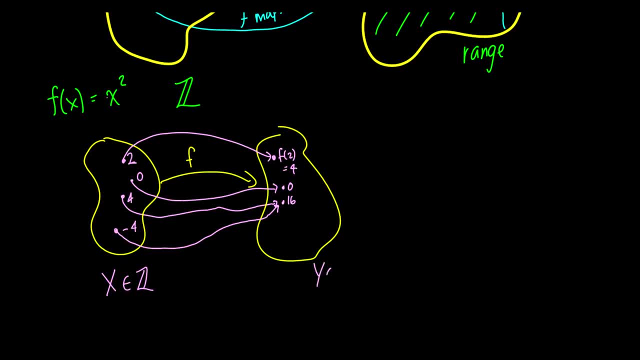 an integer and Y is an integer, then what this function does is it maps an integer to the same point. so if we say that X is an integer and Y is an integer, it maps an integer onto another integer. but what's more interesting, really, is that it doesn't just map an integer onto an integer, it maps any integer onto a. 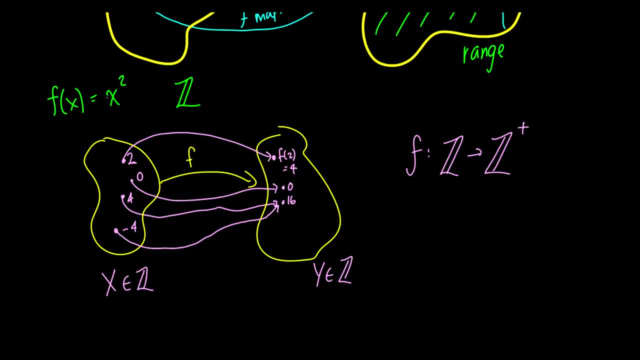 positive integer. so that's a little bit interesting. we have a function that takes an integer into a positive integer. but, more importantly, when we talk about the co domain and range, we see that the co domain is an integer and is going to be all of the positive integers. 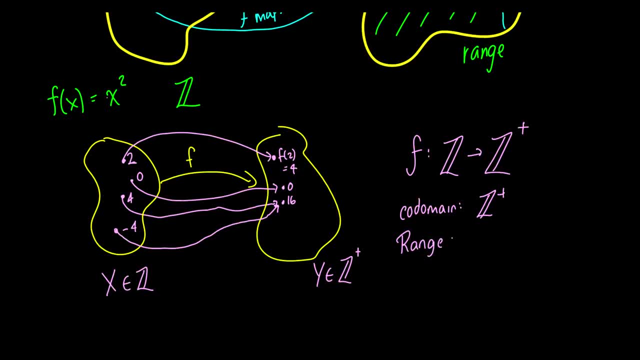 But what is the range? Well, this is a little bit more interesting, because is there any possible way I can get the number 3 from an integer by squaring it? And the answer is no. So we have nothing that maps onto 3, even though 3 is in the set. 3 is a positive integer in y. 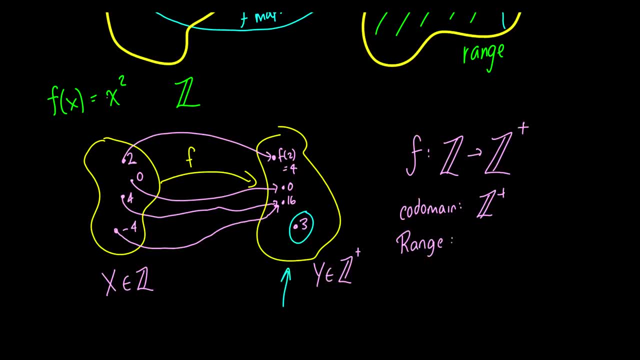 in this codomain here, But you can't get it through the function. So we say that 3 isn't in the range. In fact the range is the set of all x squared such that the square root of x is an integer. So really this kind of just described the function itself. 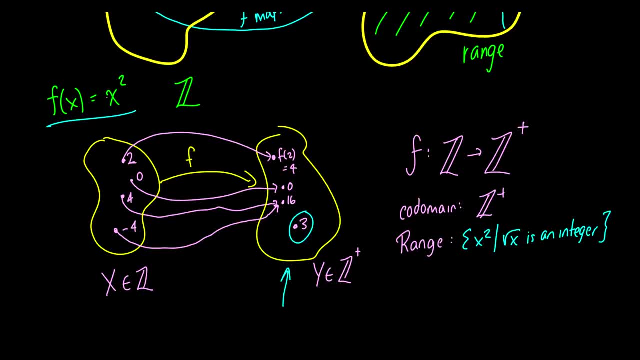 But it's important to see the contrast between the codomain and the range. So the codomain is all the possible positive integers, but the range just happens to be the integers that you can get from squaring an element in your subset x. So hopefully that's a nice concrete example. 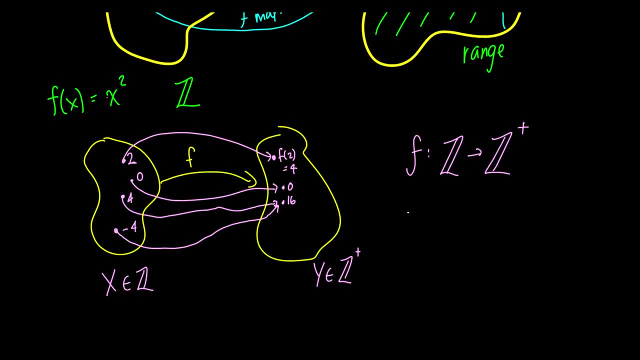 integer. but, more importantly, when we talk about the co-domain and range, we see that the co-domain actually doesn't just take an integer into an integer, but does it map. a positive integer is going to be all the positive integers, But what is the range? Well, this is a little bit more interesting. 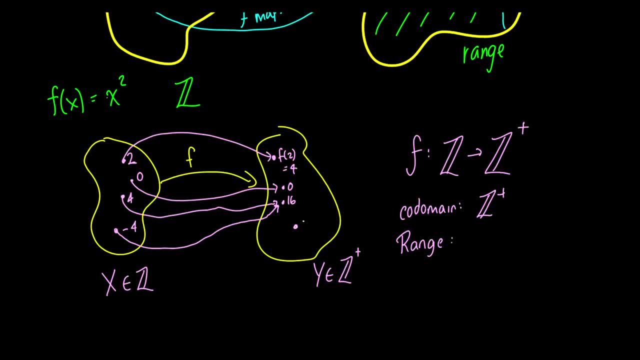 because is there any possible way I can get the number 3 from an integer by squaring it? And the answer is no, So we have nothing that maps onto 3, even though 3 is in the set. 3 is a positive integer in y. 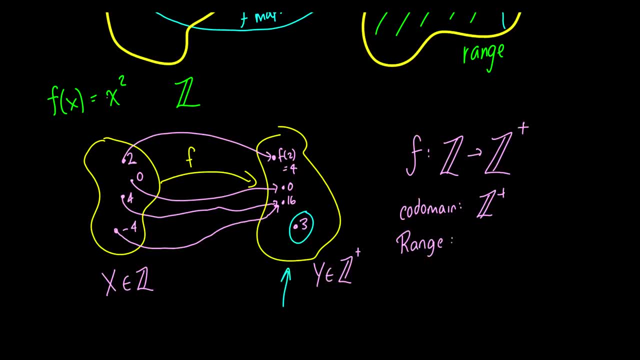 in this codomain here, But you can't get it through the function. So we say that 3 isn't in the range. In fact the range is the set of all x squared such that the square root of x is an integer. So really this kind of just described the function itself. 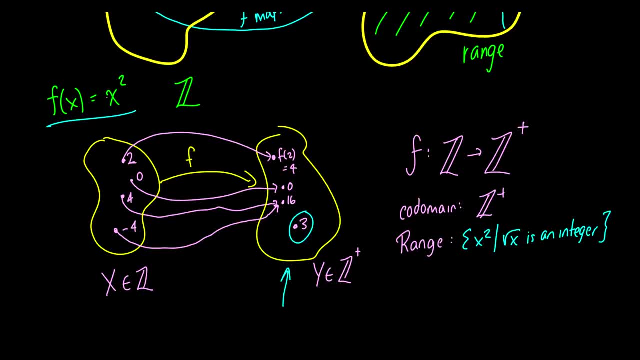 But it's important to see the contrast between the codomain and the range. So the codomain is all the possible positive integers, but the range just happens to be the integers that you can get from squaring an element in your subset x. So hopefully that's a nice concrete example. 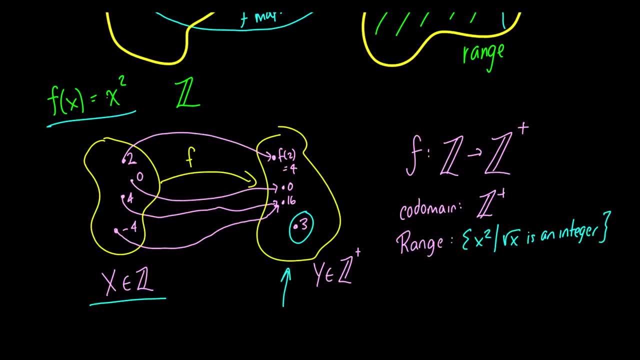 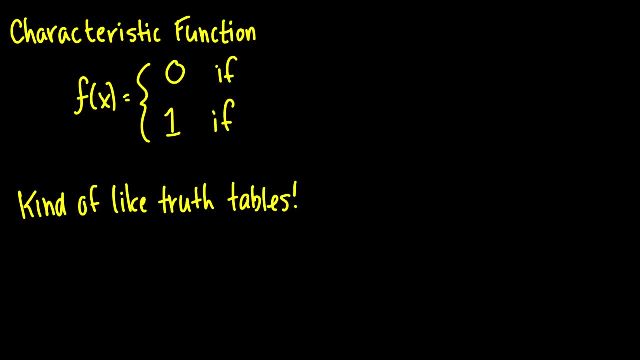 If not always, just leave your questions down there. in that section We should talk about characteristic functions because they relate to logic, a lot and set theory and pretty much everything to do with ones and zeros and Boolean algebra. This is a simple function, If you have. 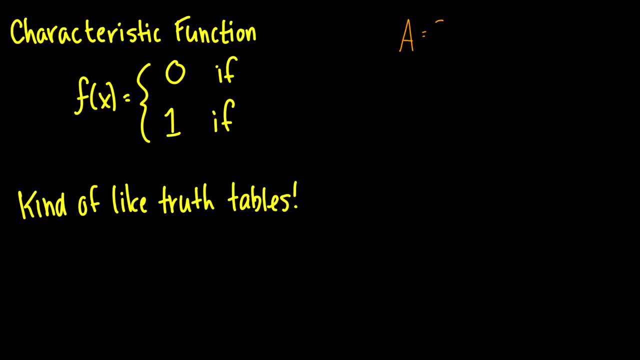 a, set A and you have a bunch of elements in there like A, B, C, so on forever. if the element x is in A, then it gets a 1.. If the element x is not in A, then it gets a 0.. 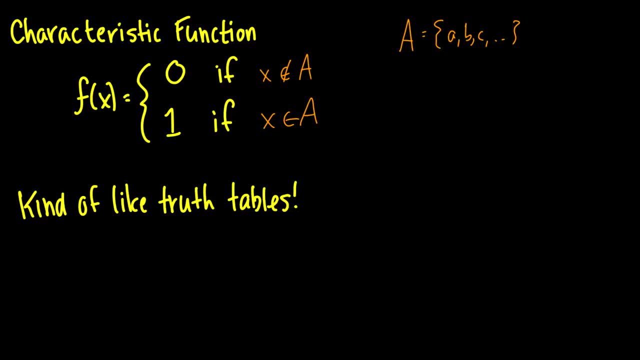 So it's basically saying: is something present? So if I say, okay, let's take the characteristic function, and what we're saying here is we have a set, I don't know. let's say the set takes an integer and it maps it to either a 0 or a 1. 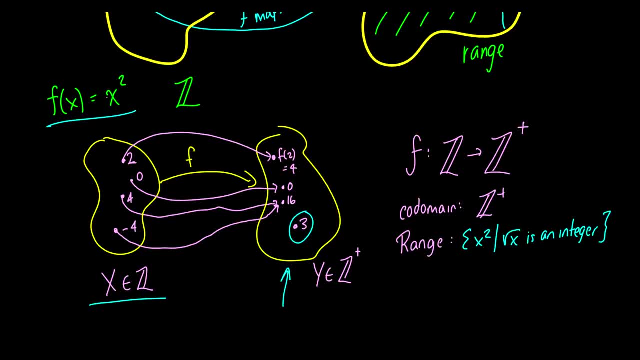 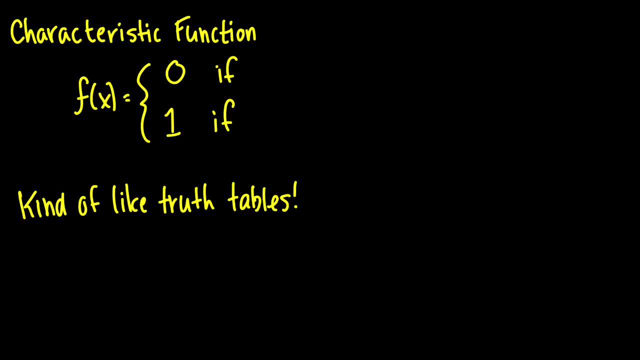 If not always, just leave your questions down there. in that section We should talk about characteristic functions because they relate to logic, a lot And set theory and pretty much everything to do with ones and zeros and Boolean algebra. This is a simple function, If you have. 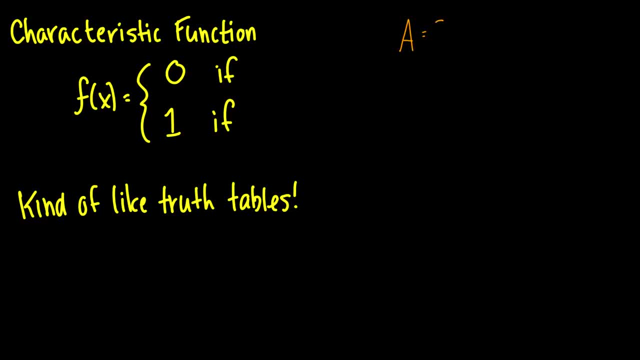 a, set A and you have a bunch of elements in there like a, b, c, so on forever. If the element x is in A, then it gets a 1.. If the element x is not in A, then it gets a 0.. 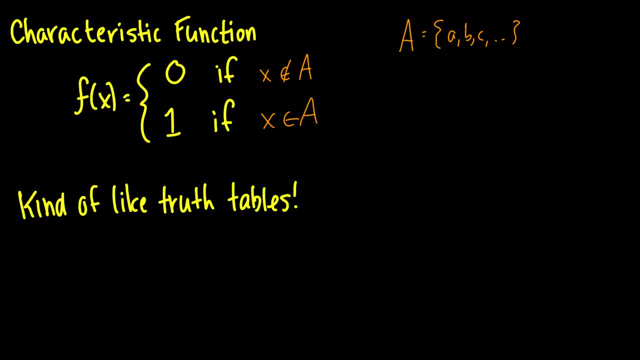 So it's basically saying: is something present? So if I say, okay, let's take the characteristic function, And what we're saying here is we have a set, I don't know. Let's say the set takes an integer and it maps it to either a 0 or a 1.. 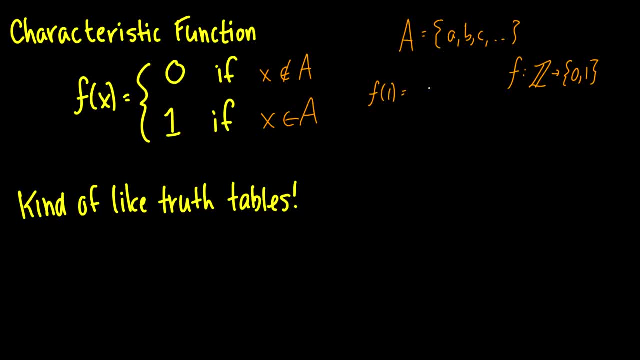 And we say, okay, is f of 1 in the set? And we say, yeah, it's in the set. What about f of 2 in the set? And we say, hmm, no, f of 2 is not in the set. Then we go: what about f of 3?? 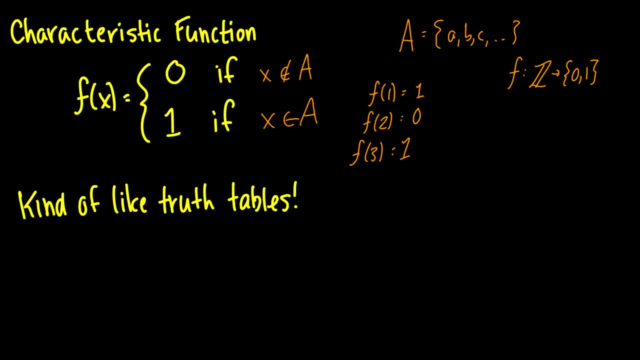 Yeah, that's in the set So we can kind of determine- not necessarily yet, but that maybe this is a function that checks if a number is odd And we can further testing it by saying: okay, well, what is f of 4?? 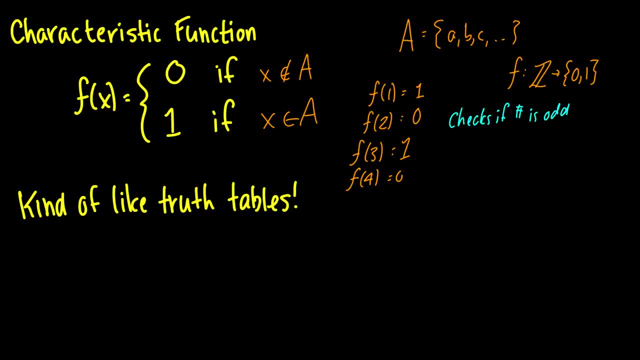 And that's 0.. So, okay, well, what is f of 4? And that's 0.. So okay, well, what is f of 4? And that's 0.. So clearly, 4 isn't in the set And you can infer a pattern's going to be like that. 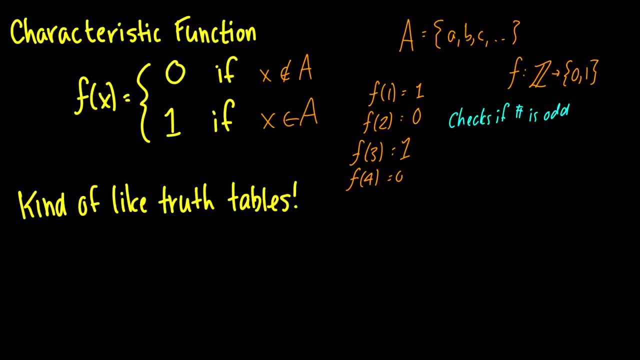 So we can say: okay, it's the function that checks if a number is odd. If it is odd, we get a 1.. If it's not odd, we get a 0.. So that's the practical application of the characteristic function And you'll see. 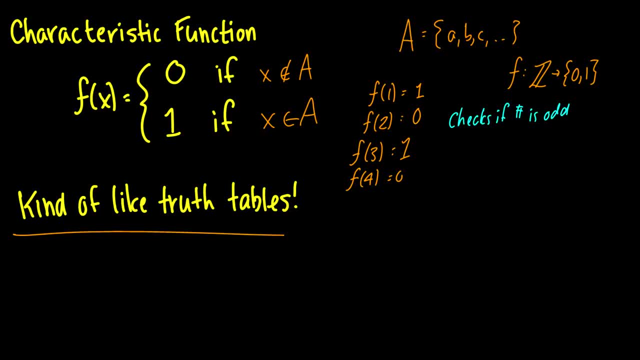 it's pretty much truth tables. I mean, if we say, okay, we have a p of x function here And we have values of x which happen to be 1,, 2,, 3,, 4, 5. What we do is we just evaluate it. So 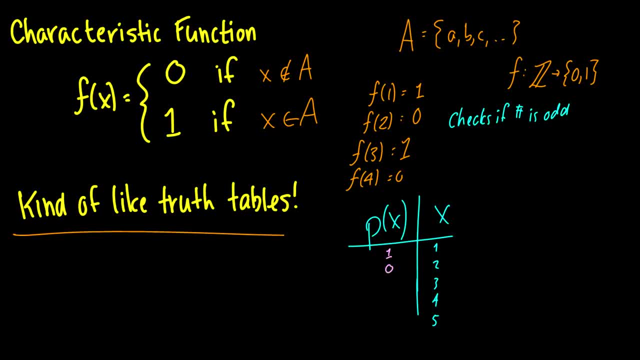 p of x. when x is 1, is going to be a 1.. When it's 2,, it'll be a 0.. When it's a 3, it's a 1.. 4 is 0.. 5 is a 1.. So on and so forth. 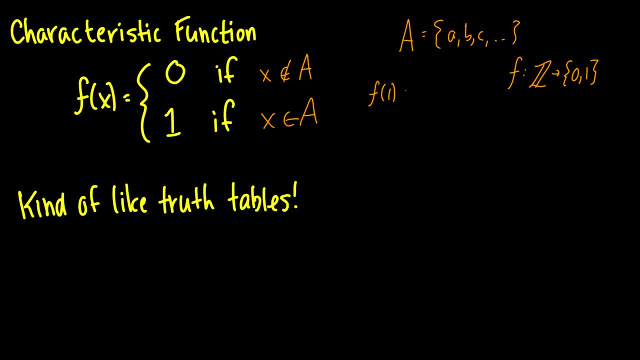 and we say, okay, is f of 1 in the set? and we say, yeah, it's in the set. what about f of 2 in the set? And we say, hmm, now f of 2 is not in the set. Then we go: what about f of 3?? 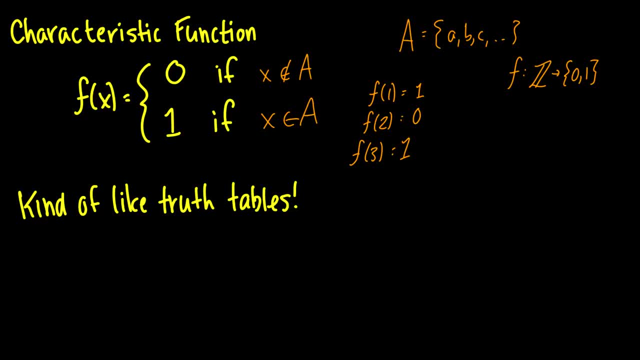 Yeah, that's in the set So we can kind of determine- not necessarily yet, but that maybe this is a function that checks if a number is odd And we can further testing it by saying: okay, well, what is f of 4?? 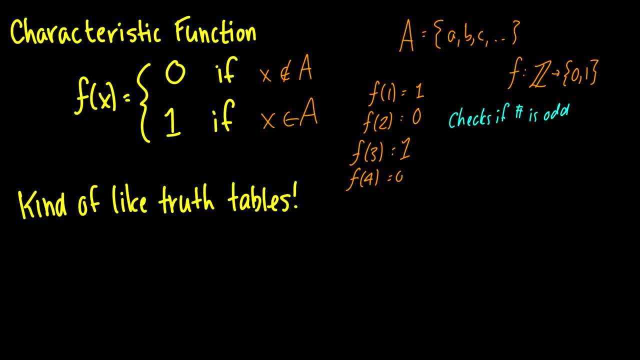 And that's 0.. So clearly 4 isn't in the set And you can infer a pattern is going to be like that. So we can say: okay, it's the function that checks if a number is odd. If it is odd, we get a 1.. 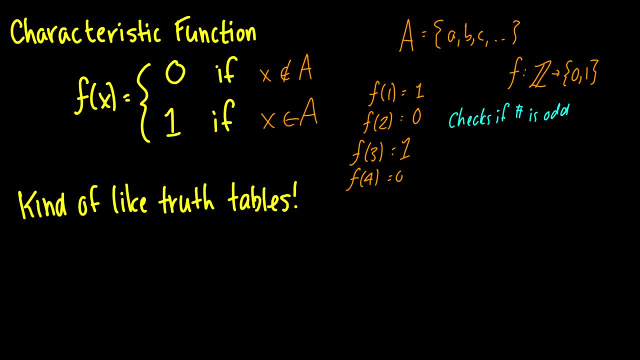 If it's not odd, we get a 0.. So that's the practical application of the characteristic function And you'll see it's pretty much truth tables. I mean, if we say, okay, we have a p of x function here. 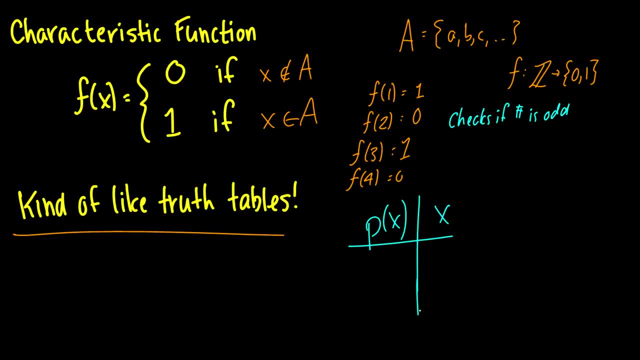 And we have values of x which happen to be 1,, 2,, 3.. 4, 5.. What we do is we just evaluate it. So p of x, when x is 1, is going to be a 1.. 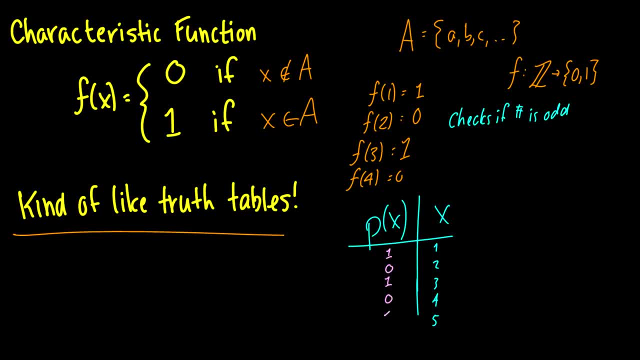 When it's 2,, it'll be a 0.. When it's a 3,, it's a 1.. 4, 0.. 5 is a 1.. So on and so forth. So this is a cool little truth table. 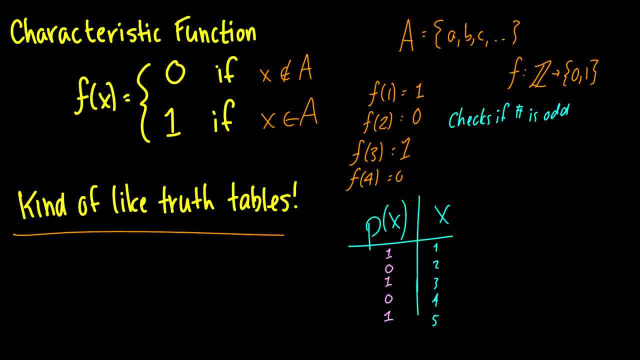 And it's pretty much the same thing. In fact, it's kind of how truth tables are made. But if you want a real nice explanation of how you get truth tables, you probably want to check out Axiomatic Logic, which at the time of this video. 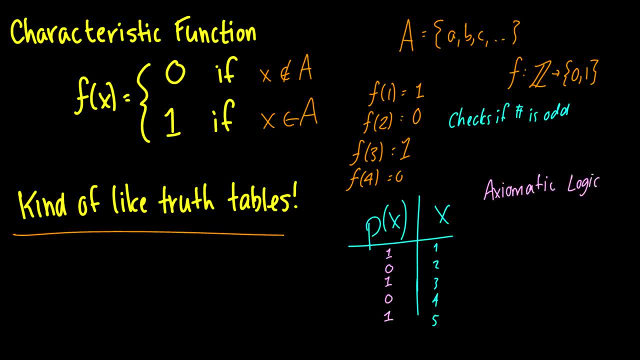 I haven't done yet, But it covers something called the Filtration Theorem, which shows you how to produce truth tables. So there should be videos online about that if you're really interested about how you make truth tables with characteristic functions. But that is another video. 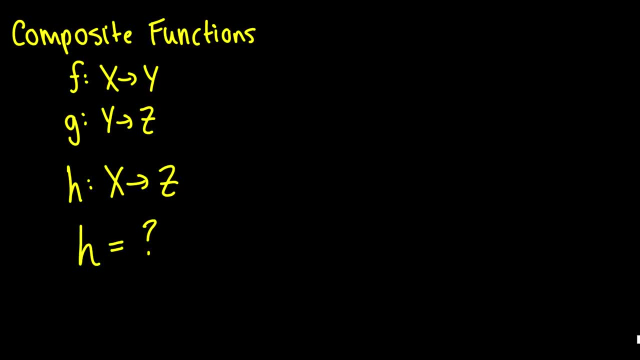 So let's talk about composite functions. I know this one's a little bit fast, but There's really not that much to it, So a lot of people get confused. So I'm just going to use some points here. This is our x. 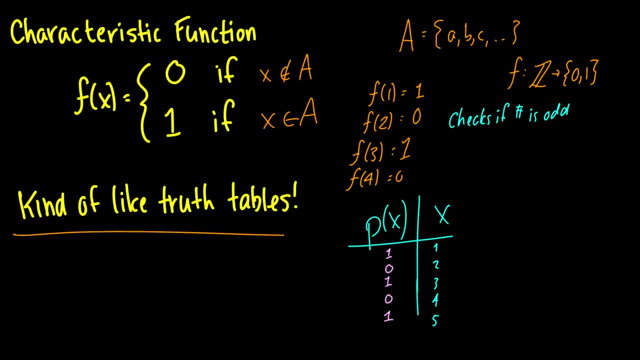 So this is a cool little truth table And it's pretty much the same thing. In fact, it's kind of how truth tables are made. But if you want a real nice explanation of how you get truth tables, you probably want to check out axiomatic logic, which 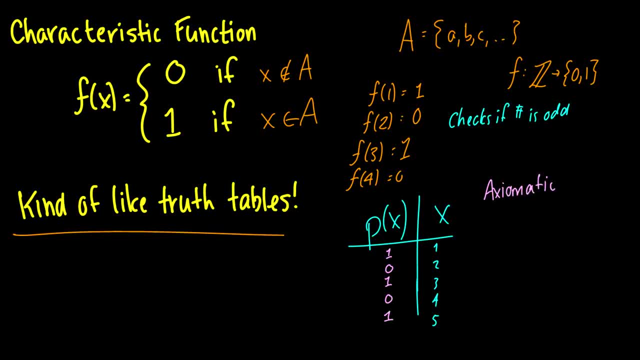 at the time of this video. I haven't done yet, But it covers something called the filtration theorem, which shows you how to produce truth tables. So there should be videos online about that if you're really interested about how you make truth tables with characteristic functions. 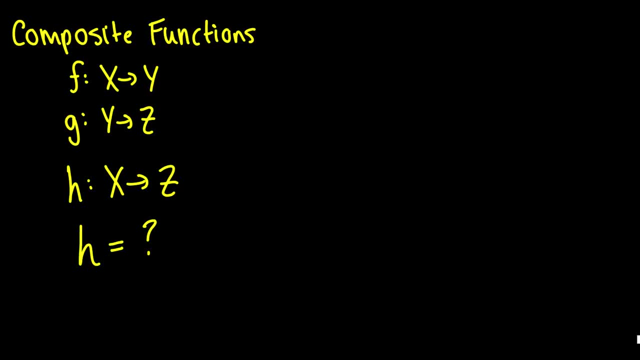 That is another video, So let's talk about composite functions. I know this one's a little bit fast, but there's really not that much to it. A lot of people get confused, so I'm just going to use some points here. 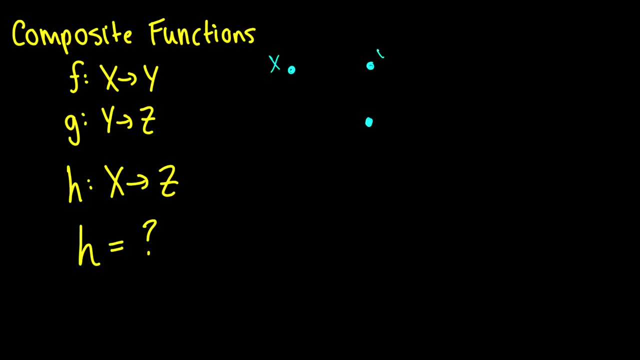 This is our x, this is our y, this is our z. These are sets okay. So I'm going to draw arrows representing what's going on here. So x goes to y, and this is done by the function f, y goes to z, and this is done by the function g. 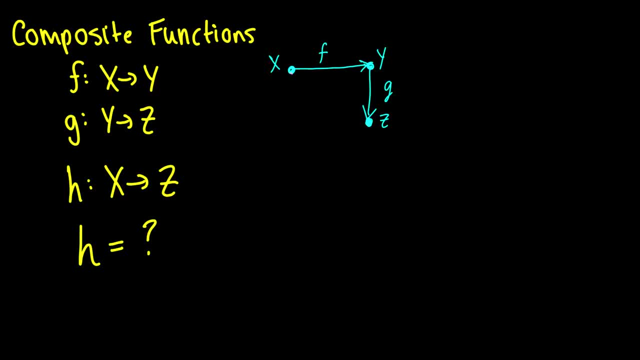 We have this other function, h, which takes x to z, and this is called h. Now, clearly we see a relationship between these functions. We see that the function f and the function g are similar to h. In fact, if we do both of them, they're going to be similar to h. But the question is: what is the order? 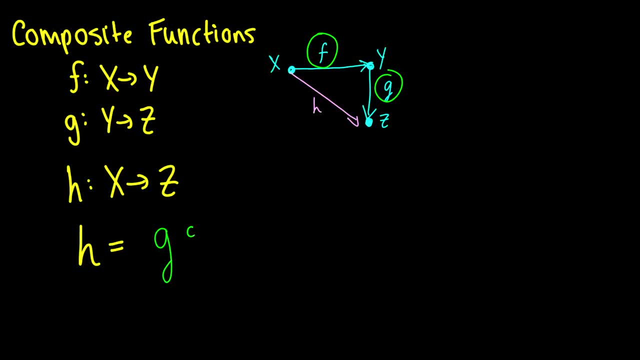 And we say that the order of h is g, with the composite function f, which I know seems a little bit counterintuitive, since you're saying: why are we doing the last one first? It doesn't make any sense. Well, this is the same thing. 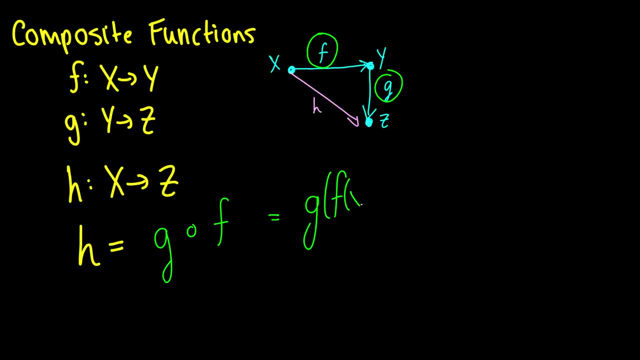 as saying g of f, of x. So what this does is first this inner part takes a function from x to y, and then this outer part takes the function from y to z. So sort of by transitivity it then results in taking the function. 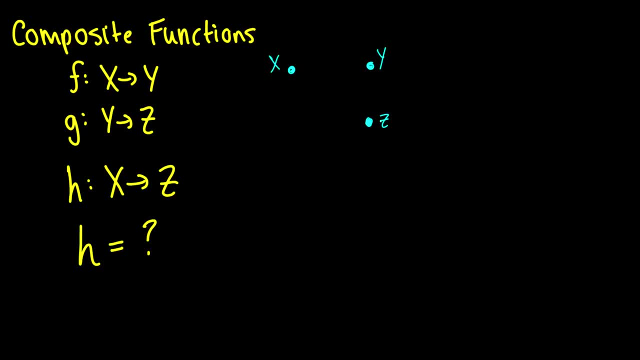 This is our y, This is our z. These are sets okay. So I'm going to draw arrows representing what's going on here. So x goes to y, and this is done by the function f. y goes to z, and this is done by the function g. 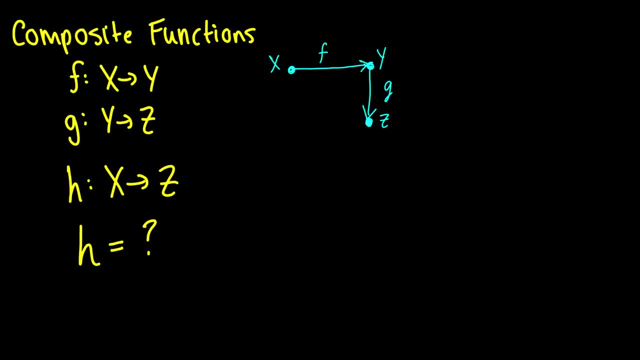 We have this other function, h, which takes x to z, and this is called h. Now, clearly we see a relationship between these functions. We see that the function f and the function g are similar to h. In fact, if we do both of them, they're going to be similar to h. 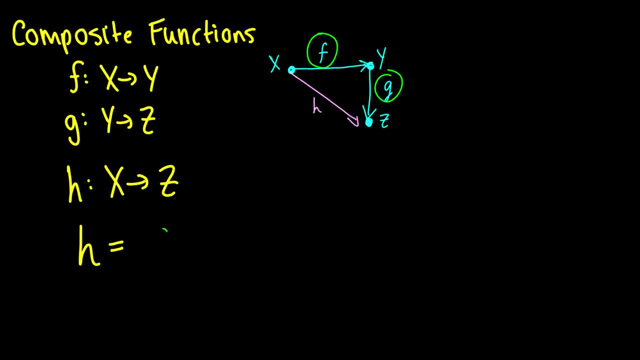 But the question is, what is the order? And we say that the order of h is g, with the composite function f, which I know seems a little bit counterintuitive, since you're saying: why are we doing the last one first? 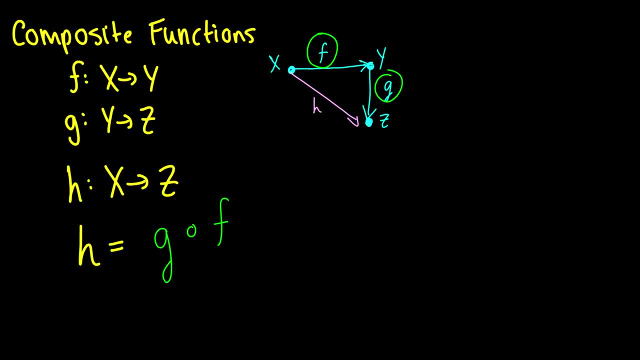 It doesn't make any sense. Well, this is the same thing as saying g of f of x. So what this does is: first this inner part takes a function from x to y, and then this outer part takes the function from y. 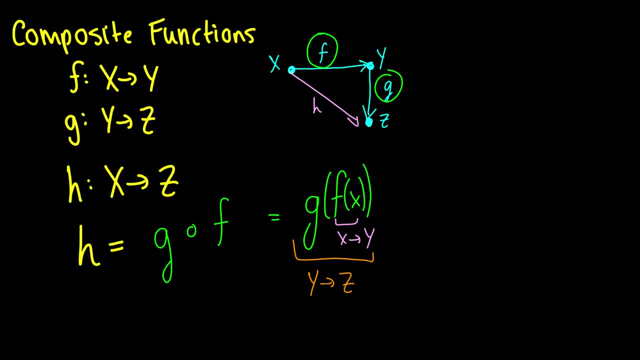 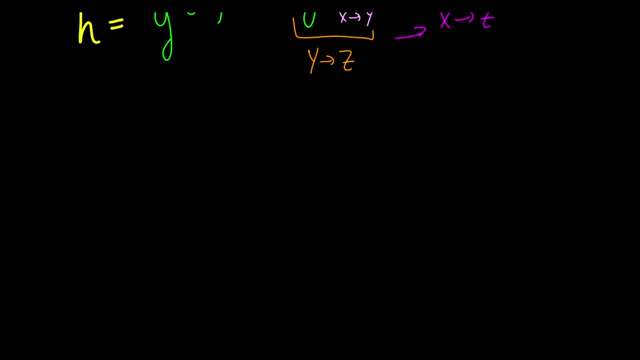 to z, So sort of by transitivity it then results in taking the function from x to z, which is the same thing that h does. It's just a nice composite function. So here's a little interesting question. Suppose I have. I don't know, let's do some dots here. 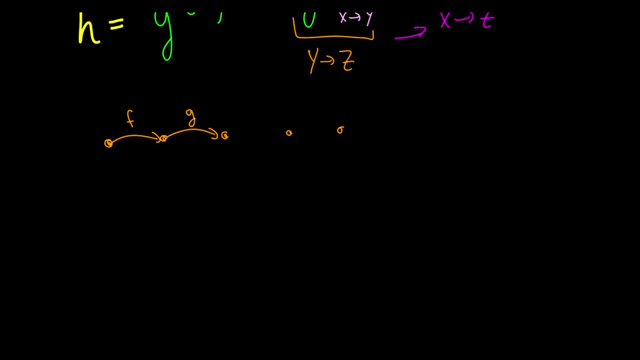 and this is f, this is g, this is h, this is j and, of course, we're going from x to y, to z, to w, to v. What is the composite function that takes us directly from x to v? And we're going to call this function k. 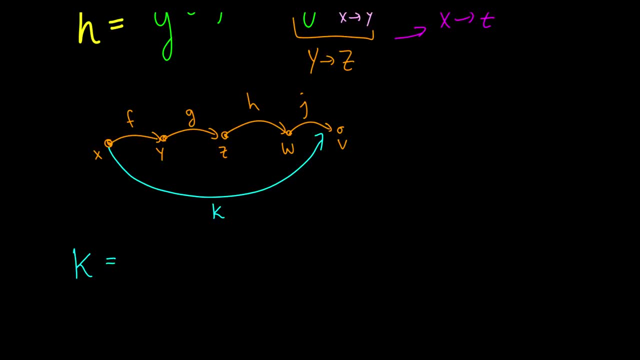 Can we define k as a composition of functions? And well, this is actually very simple. We simply just take the functions in reverse order. So this is j, dot h, dot g, dot f, which we can say that this is just j of h, of g, of f, of x. 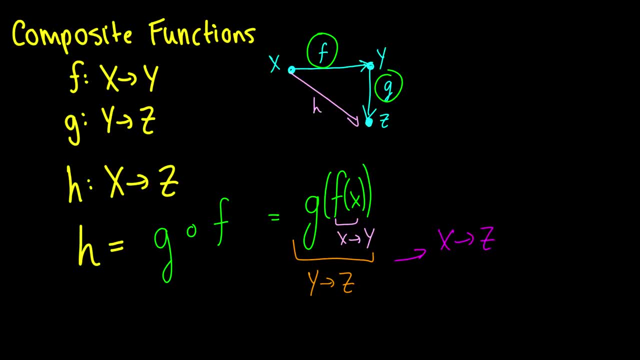 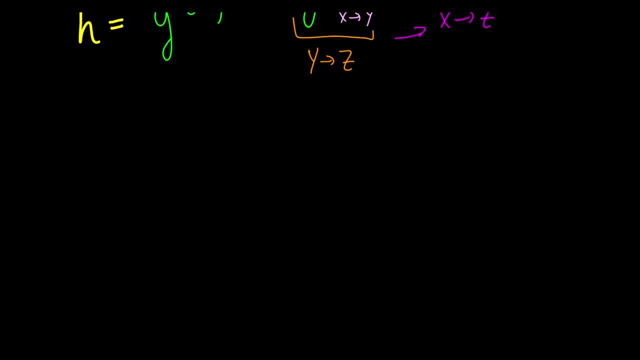 from x to z, which is the same thing that h does. It's just a nice composite function. So here's a little interesting question. Suppose I have- I don't know, let's do some dots here- and this is f, this is g. 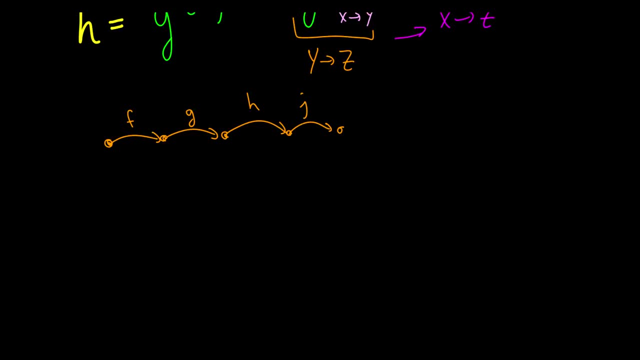 this is h, this is j and, of course, we're going from x to y, to z, to w to v. What is the composite function that takes us directly from x to v, and we're going to call this function k? Can we define k as a composition of? 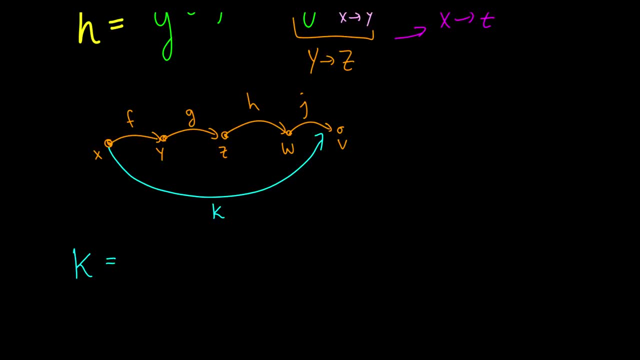 functions. And well, this is actually very simple. We simply just take the functions in reverse order. so this is j dot h, dot g, dot f, which we can say that this is just j of h, of g, of f, of x. 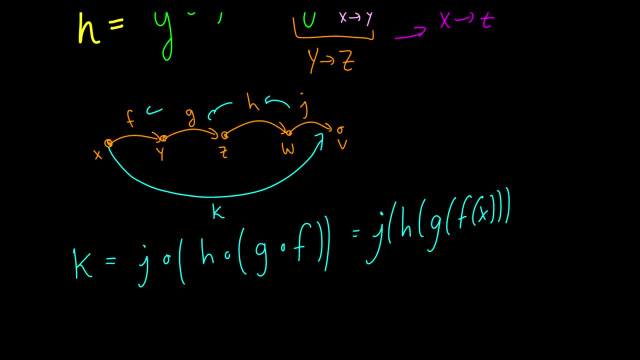 So we have three brackets. three brackets When we evaluate this function. really, this just becomes j of h of g of x, sorry, g of y, which becomes j of h of- let's put this down a little bit- j of h of z. 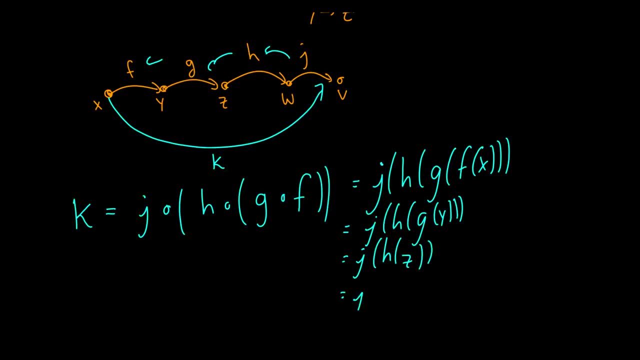 which is just j of w, which simply outputs as v. So that's kind of cool. In fact, we see that k took x to v, and if we keep doing these functions we do see that we actually end up at v. so our composite function is: 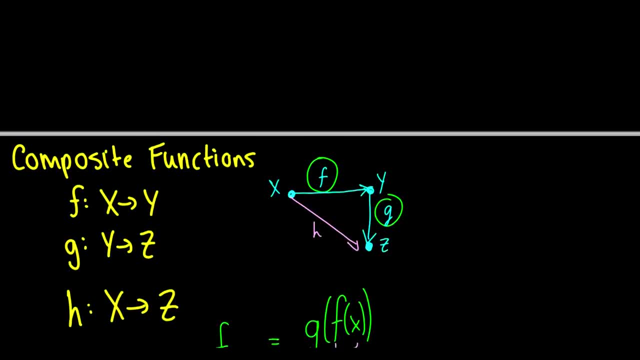 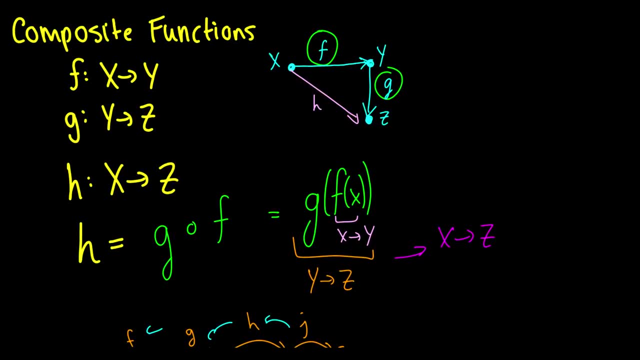 fine. So that was a quick and dirty introduction to composite functions. I know some courses will go a lot more in-depth to them. You'll have to do some proofs. If there's demand for a proof video, I'll do some proofs. but